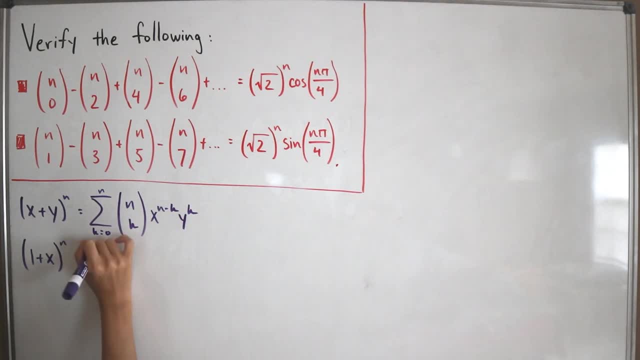 power n, and so that's equal to the expansion over here. n k is equal 0 of n. choose k. so if I plug in for x is equal to 1 over here, so it's 1, so it's always just going to be 1, so that actually just. 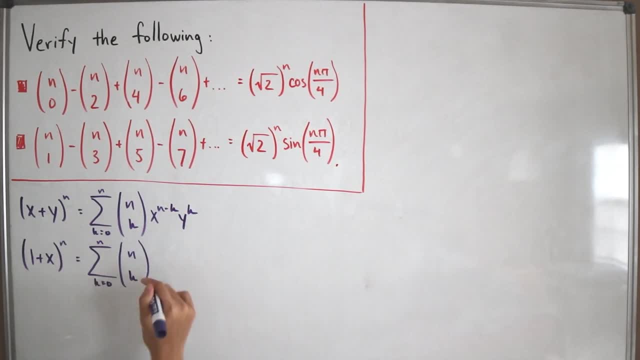 vanishes, quote-unquote, then continuing forward. So that means I have x to the power k right here. okay, so let's actually expand this out. so I have. the expansion is written as follows: so we have n, choose 0, then with x to the power 0, which is just. 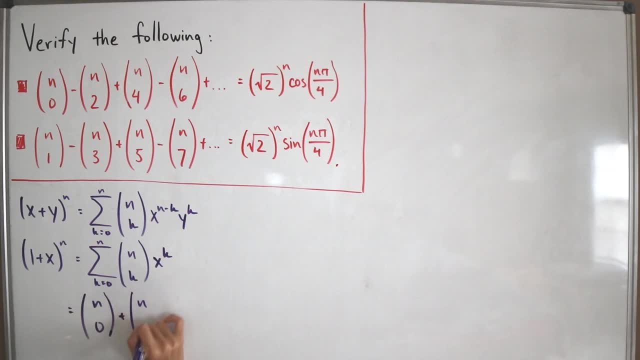 1, then I add this with n- choose 1, then x to the power 1, then plus n- choose 2, then x- square, keep going on, so on, so forth, and so we end off with n- choose n, then multiply with x to the power n. that's the expansion we have so far. so let's actually substitute something for x over. 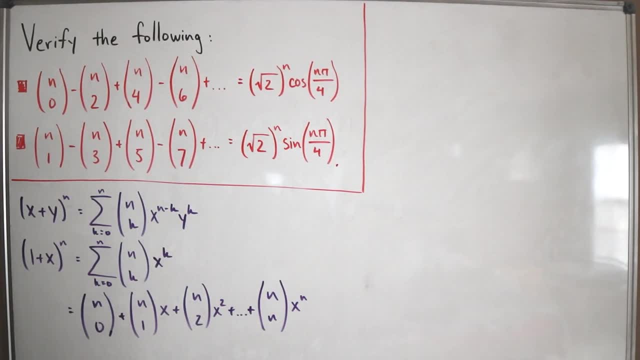 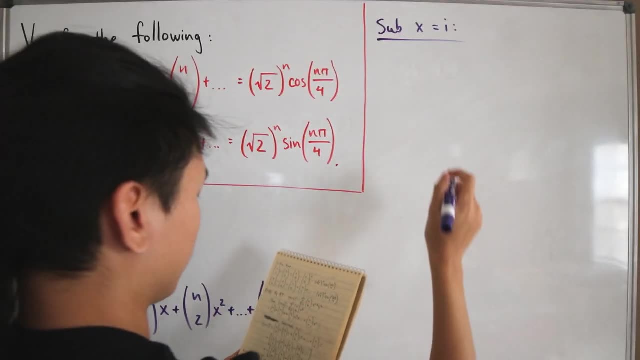 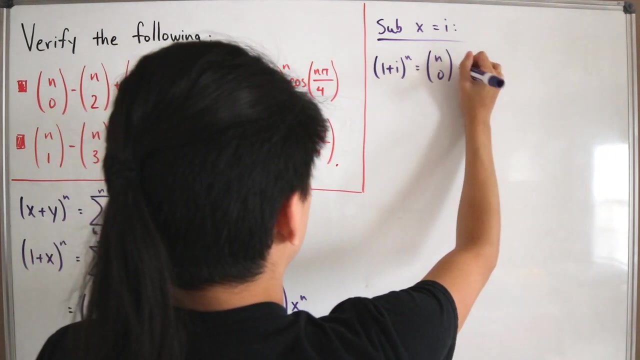 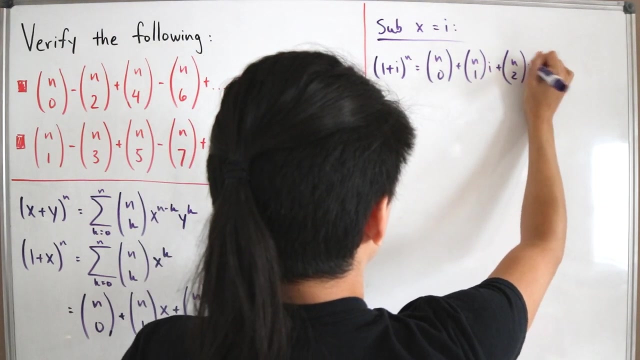 here. why don't we actually substitute x equals i, lowercase i? let's put this over here: sub x equals i, and so then we'll have this following expansion over here. so we have 1 plus i to the power. n is equal to just n. choose 0, then plus n. choose 1, then times i plus n. choose 2, then i square. 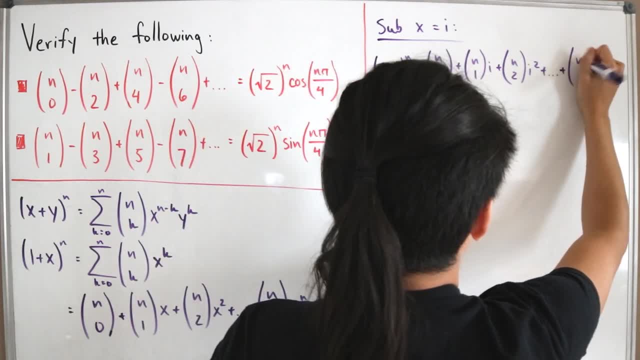 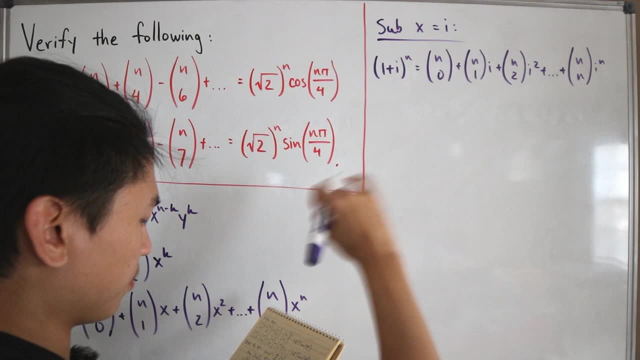 and so on. we end on the implication of n to the power i, with x to the power. 2 is equal to n, and then i to the power n. so even with this, we keep going on, so on, so forth. so ending's off with n, choose n, and then i to the power n, and so everything is with the imaginary unit i. so 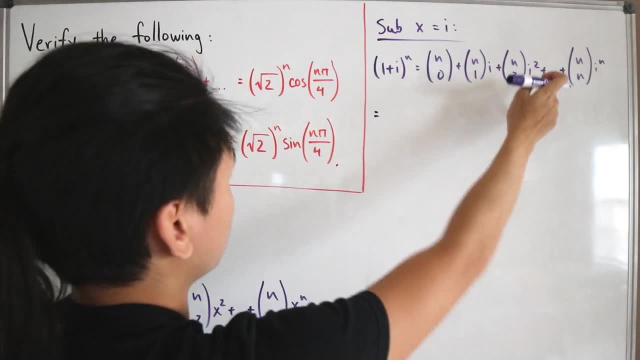 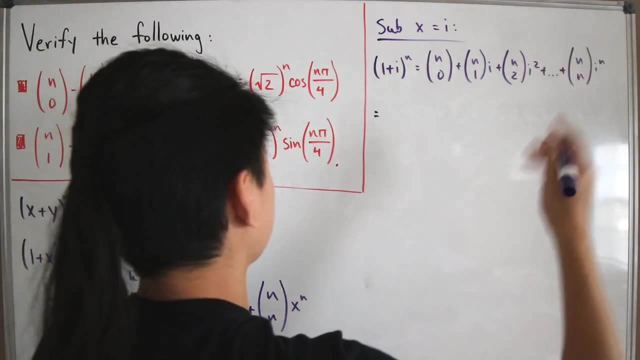 that means we'll have to separate everything from the reals and the imaginary parts. so let's actually do that. so interestingly, this is not that difficult to see- that anything with i square, i to the fourth, or even n to the zero is just on its own. those are the real parts. i square is always. 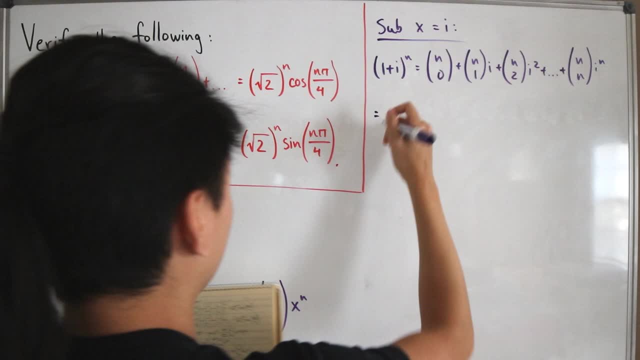 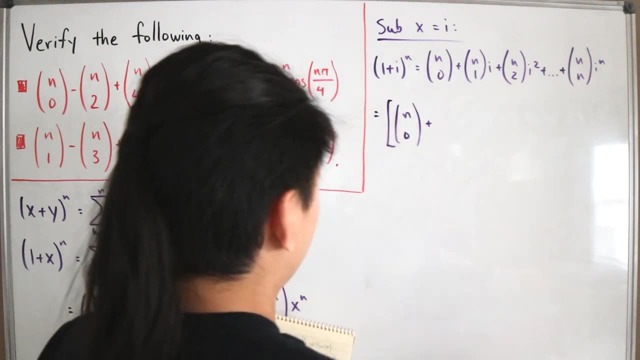 going to be equal to negative 1, then i to the fourth. so every with the evit indexes is going to one or positive one, but that's still considered part of the reals. So that means right here we have n choose zero. then add this with: well, rather subtract, because I have, i square So that 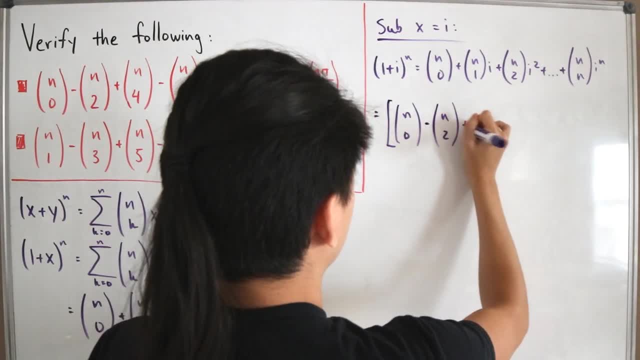 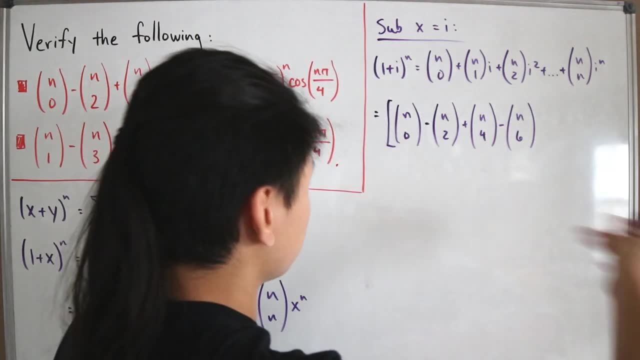 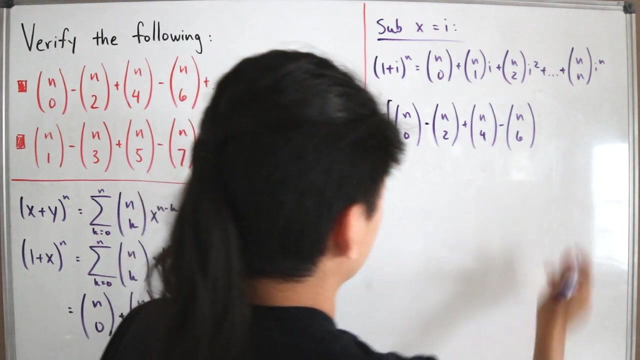 means: subtract n- choose two, then plus n- choose four, then subtract n- choose six, then plus n- choose eight. minus. It alternates for the even indices. Okay, so we can just cut that point off here. Well, let me at least add the ellipses, so it actually continues on infinitely for the evens. 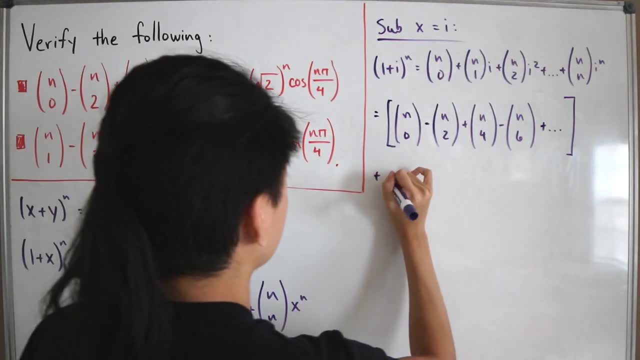 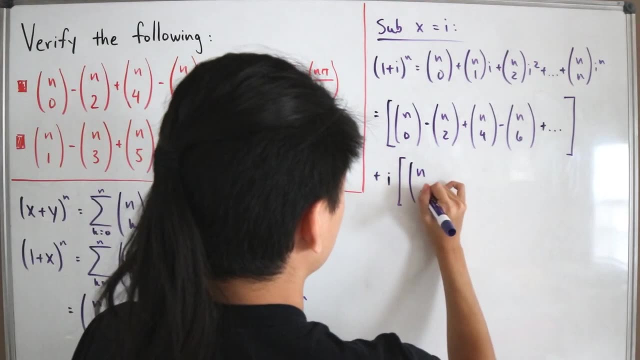 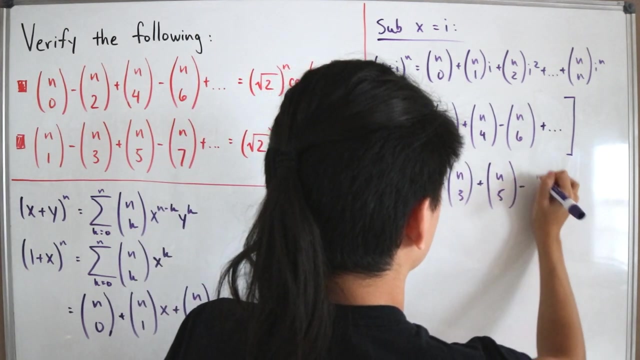 And we do the same thing, but now this is associated with the imaginary unit i and you can see that it's going to everything in terms of the odd indexes. So n choose one, then subtract n choose three. add this with: n choose five, subtract n, choose seven, then follow the ellipse. 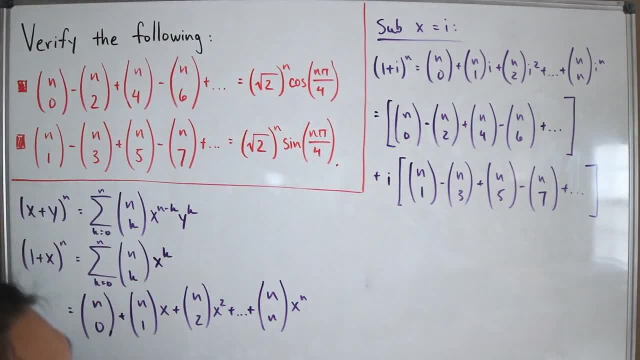 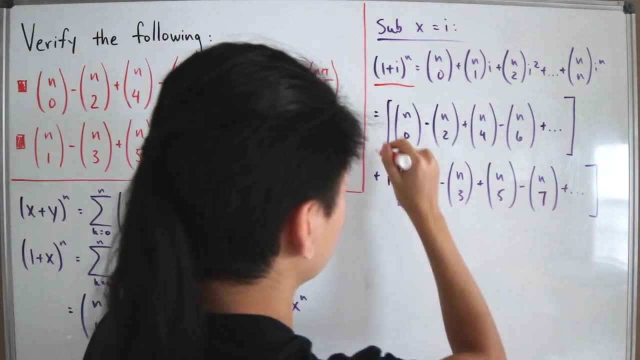 again, keep going for infinitely, So okay, So let's verify that so far, that the left-hand side one plus i to the power n so far is equal to this following expansion over here. So what's nice is that let's actually expand the left-hand. 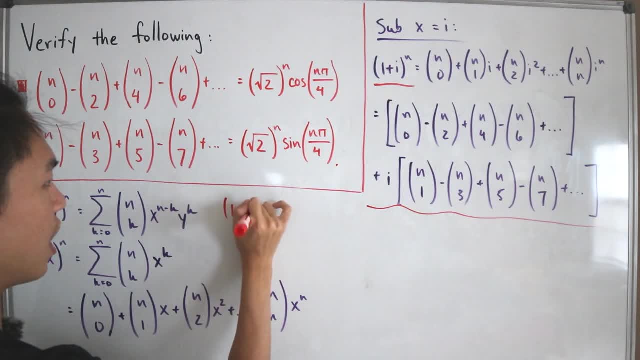 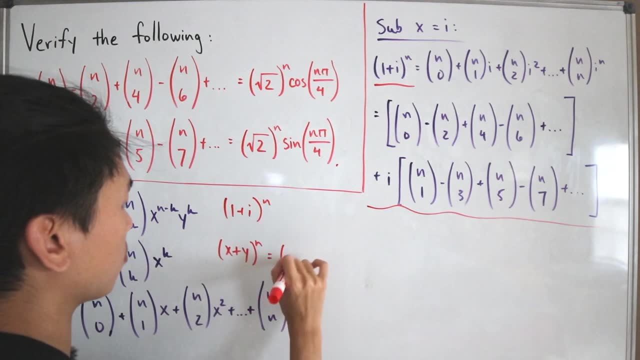 side in terms of polar form. So one plus i to the power n. So I guess it's worth noting that specifically x plus y to the power n is written as the polar form: r times e to the power i, beta then to the power n. So let me actually take that part out and then put it into the polar form. 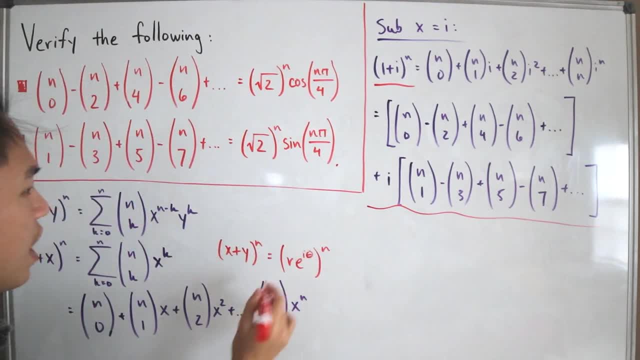 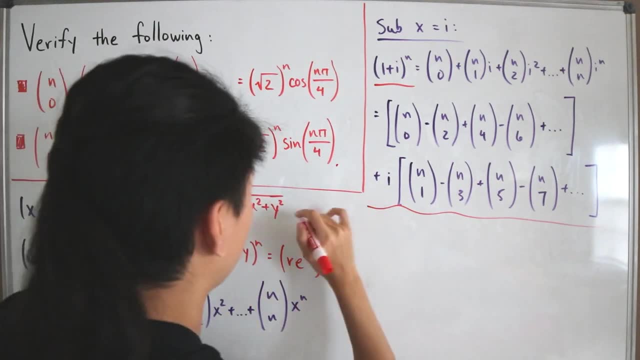 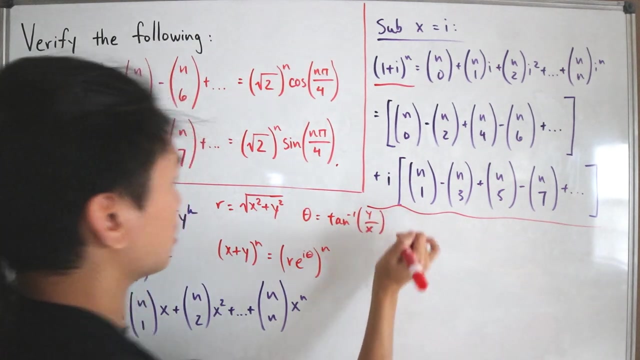 So that's supposed to mean that r is equal to our modulus, the radius x squared plus y squared, And then our theta over here is, of course, going to equal to the inverse tangent of y divided by x, data being our argument in terms of. we're looking at the complex plane. So from here now let's. 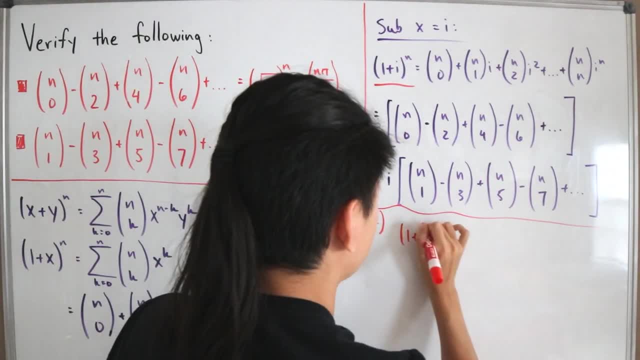 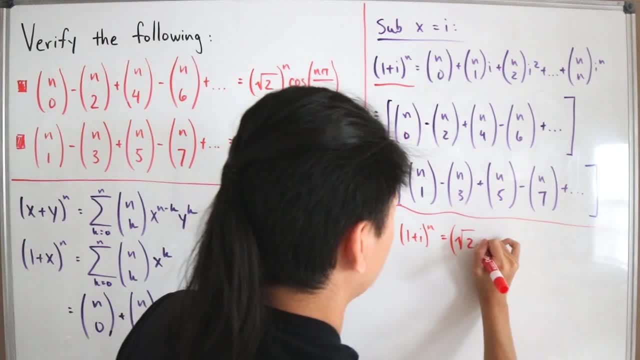 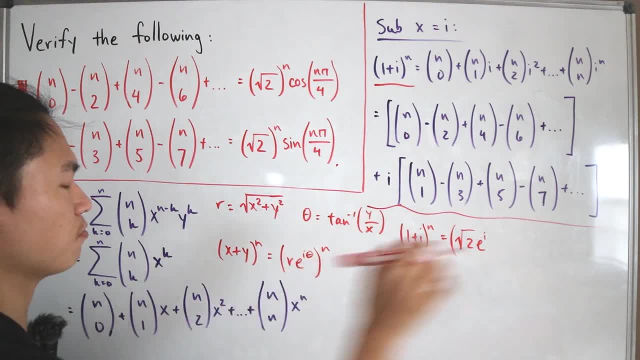 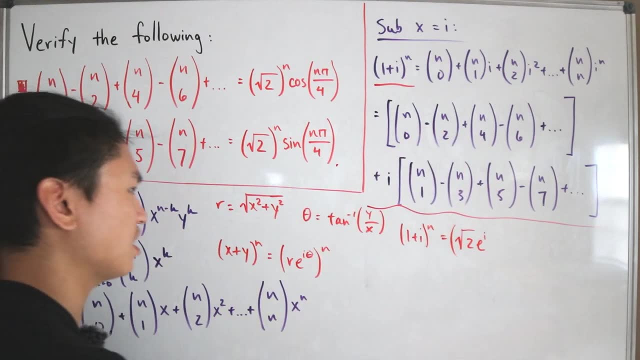 at this in terms of how this is graphically put in. So it goes to the left or it goes to the right one, and then one unit up for an imaginary, So you can see where that argument forms, that it actually forms a 45 degree angle, aka that's pi over four. and then to the power n. 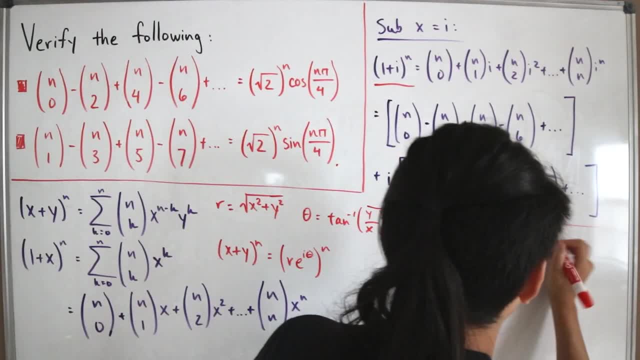 Okay, And then keep going expansion further, just to distribute the n over here. So I have that this is square root of two to the power n, then multiply with e to the power i times pi, times n divided by 4.. Then if I expand this out, of course with using Euler's formula, so that's. 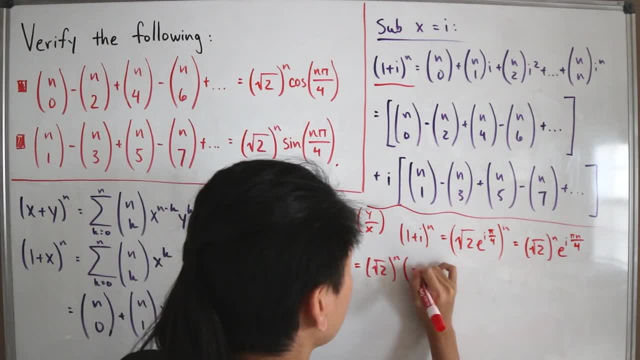 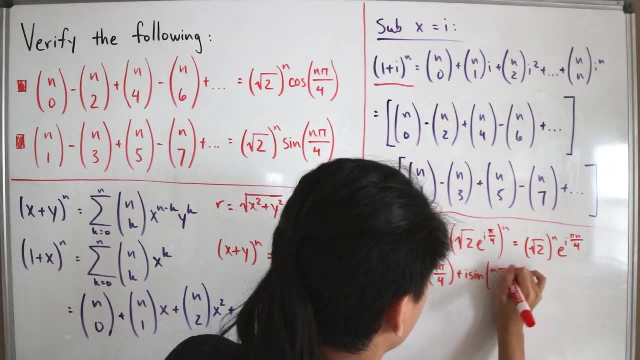 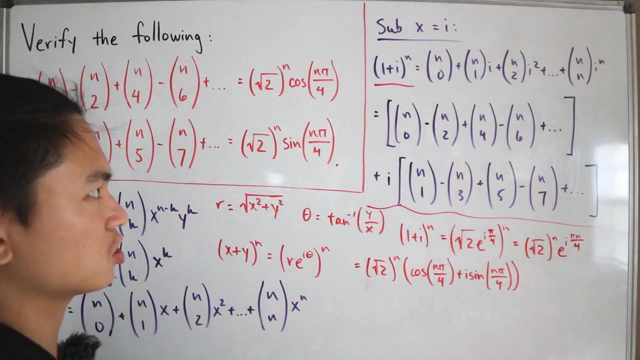 another way, saying the square root of 2 to the power n, then multiply with cosine of n pi 4, and then plus i times sine of n pi 4.. And so from here we see that this left hand side is equal to this expansion over here. so the last part, really generally, is just to now equate the real and 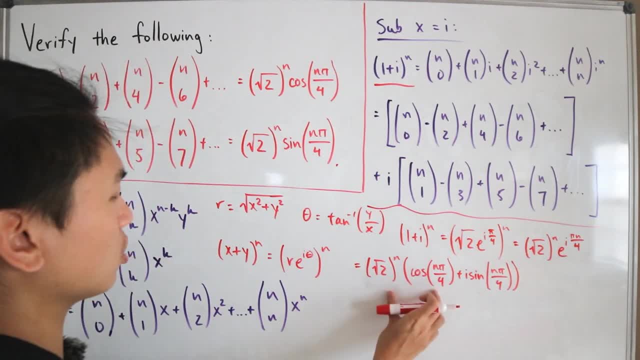 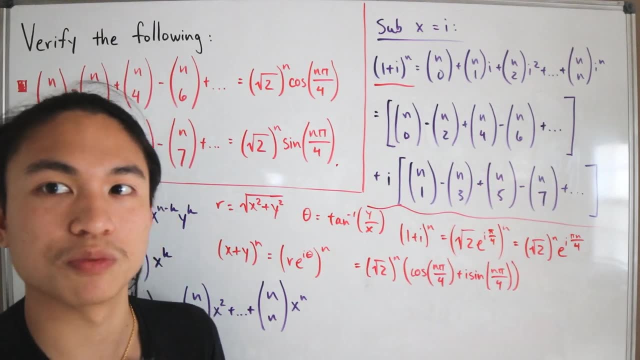 imaginary parts. So the real part being is that this associated with cosine is going to equal to this real part and then the imaginary is going to equal to this part and actually, as I said, that actually completes the proof because it takes some. it's again equating. we actually did everything in 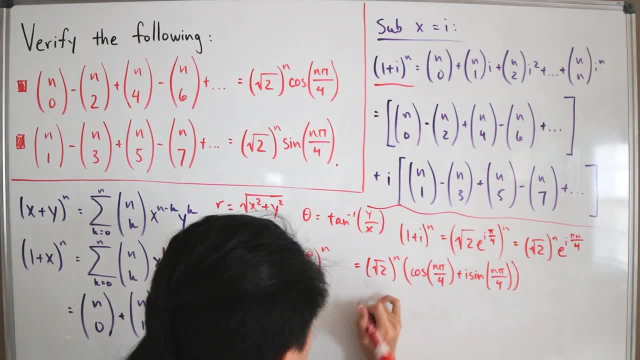 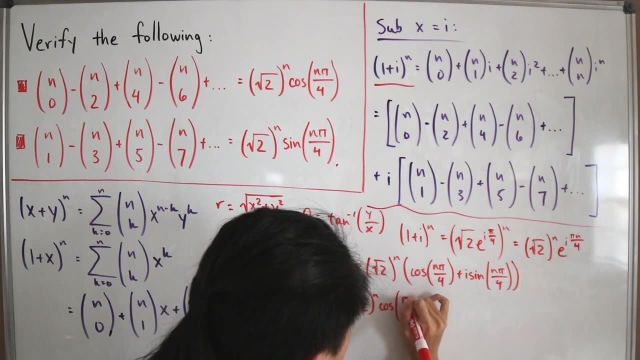 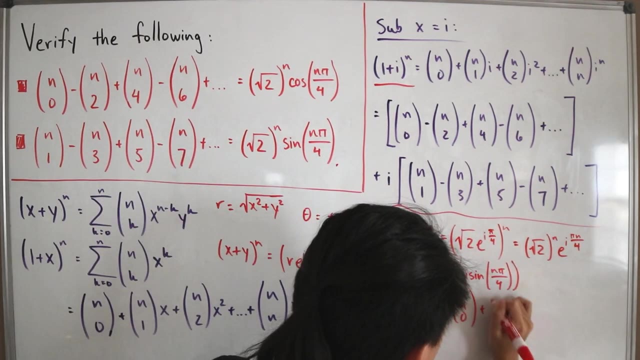 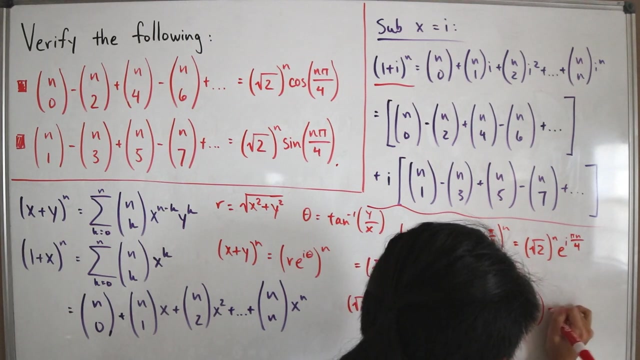 one go instead of having to do two separate proofs. and so therefore, that concludes that the square root of 2 to the power n cosine of pi times n divided by 4, is indeed just equal to you. n choose 0 plus or minus, minus. n choose 2. add this with n choose 4, and then subtract n choose 6. 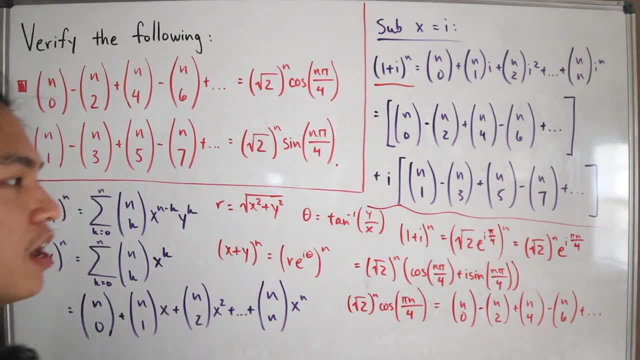 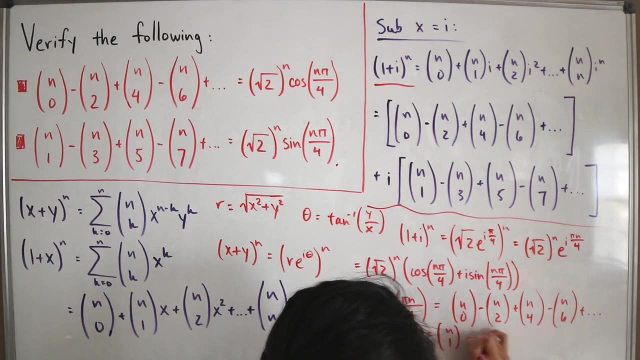 so on and so forth. so that's actually one side done. and then the other is that square root of 2 to the power n, times sine of pi, times n, divided by 4, is equal to just everything in terms of the odd indexes, and choose 1 minus n, choose 2.. 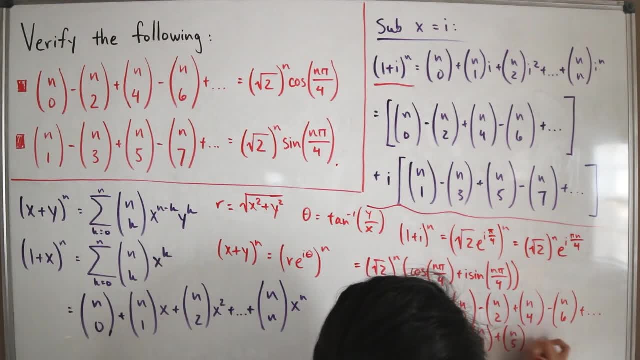 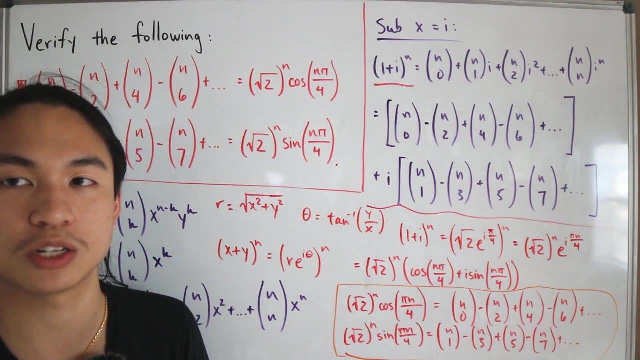 choose 3 plus n, choose 5 minus n, choose 7, then so on, so forth, and so that actually completes our proof for verifying these two identities over here, just like that. and so there we have it. as simple as it is with the nice and even with the nice relationship between terms of both the binomial. 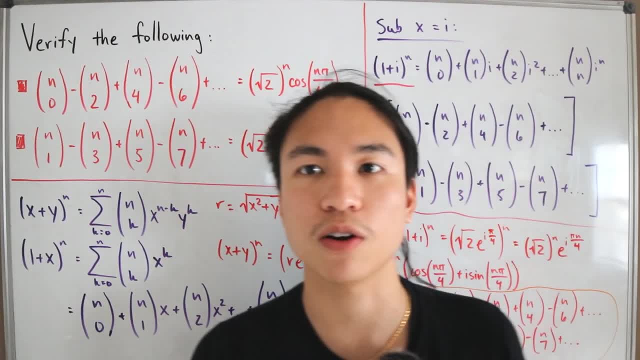 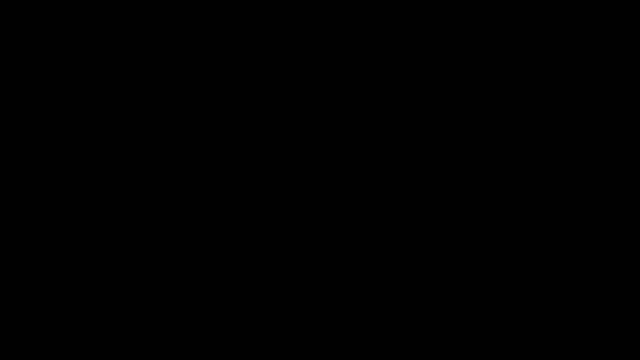 coefficients, with complex numbers and, of course, with trig functions associated with that together. so yeah, that's a pretty cool, if you ask me.